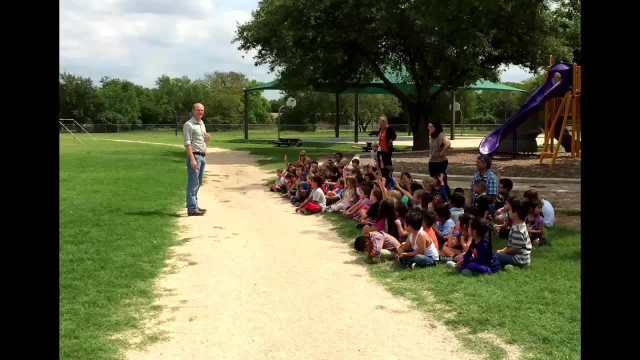 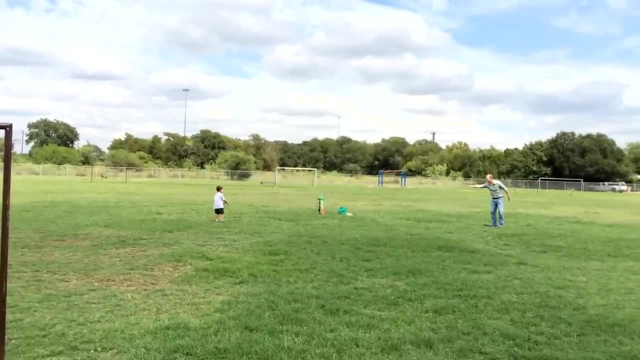 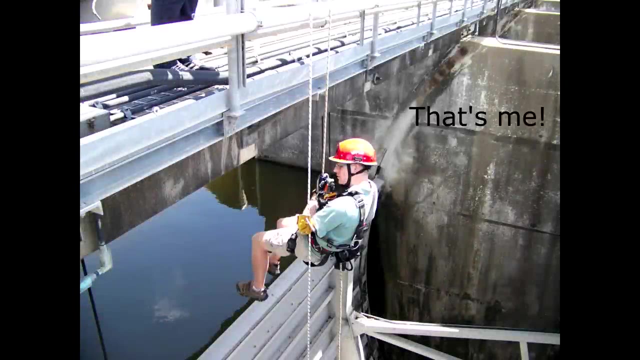 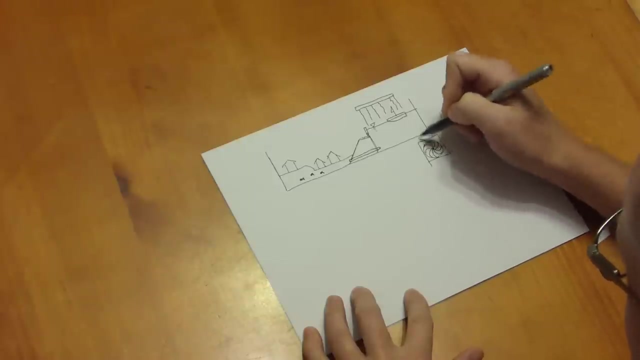 And I really enjoy this because I like what I do and it's a fun challenge to try and make it interesting to young people. I practice mainly in the field of dams and large hydraulic structures, So this year I wanted to build something to illustrate some fundamental concepts of water management. 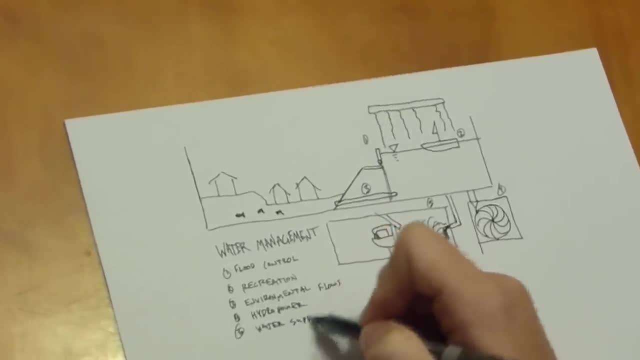 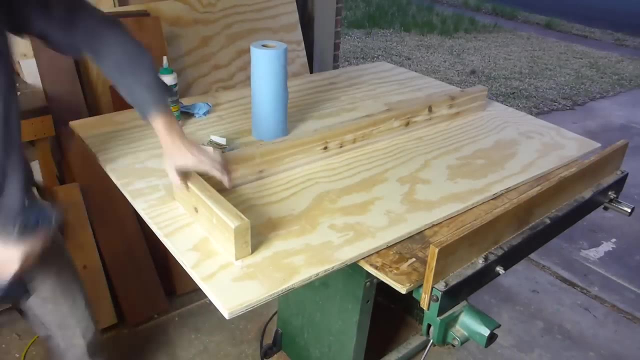 My idea is to construct a model of a dam and reservoir, kind of in the style of a children's science museum exhibit. I cut out this piece of three-quarter inch plywood and then rounded over all the edges. Then I screwed on all the cedar two-by-fours. 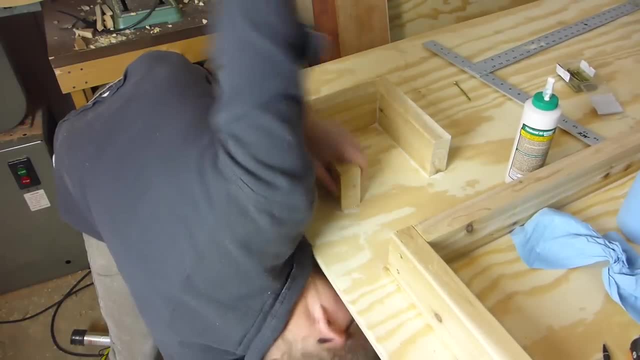 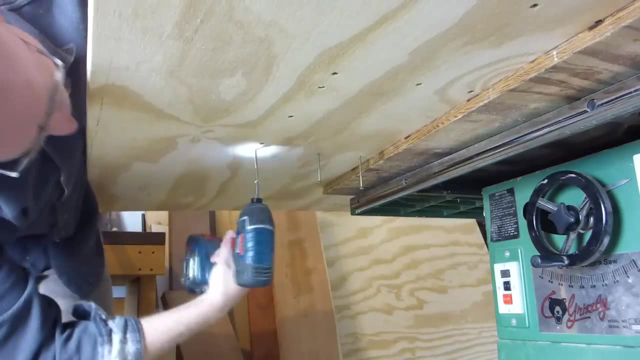 I'm using type on three here, which is a waterproof glue, although it's not really designed for submerged applications, But this is only intended to be the last line of defense against leaks. It's also a little chilly out in the shop this week. 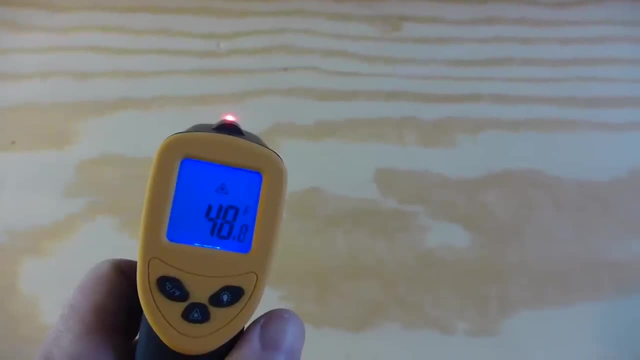 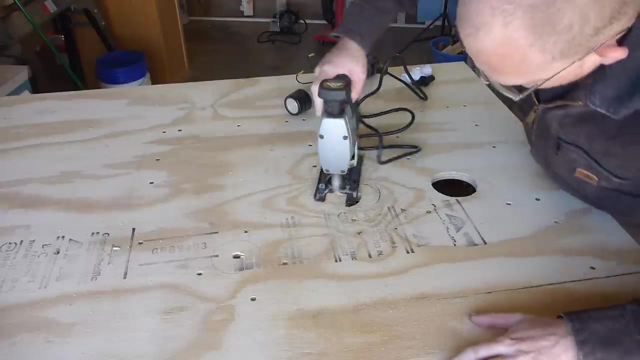 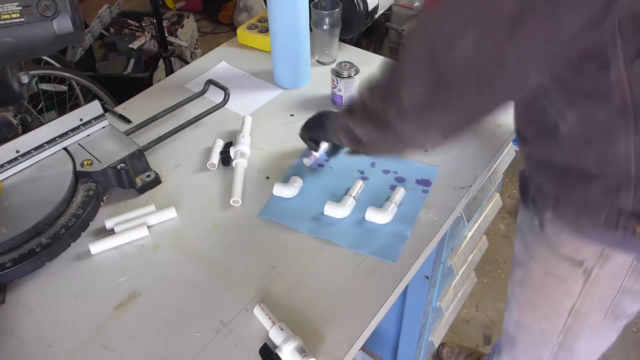 The bottle says: keep it above 45, and it's just about 50 now, So I'm hoping it stays that way for at least a few more hours. while the glue dries. I cut some windows for the water, I drilled holes for the valves, drilled holes for the pipes and started on some of the plumbing. 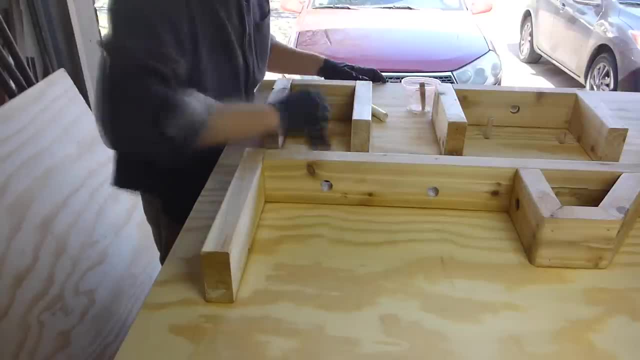 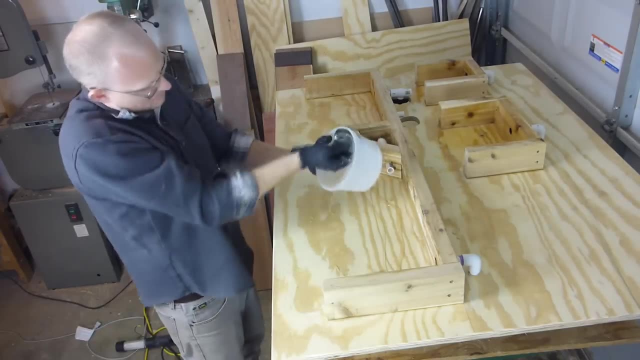 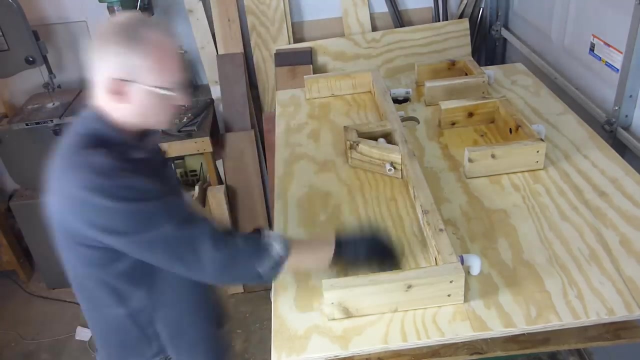 Then I coated all of the surfaces which would be getting wet with marine grade epoxy. The goal here is to prevent leaks and keep the wood from becoming saturated, which might cause it to swell or mold or just be too weak. I've never built a wooden boat before, but I think this is how they do it. 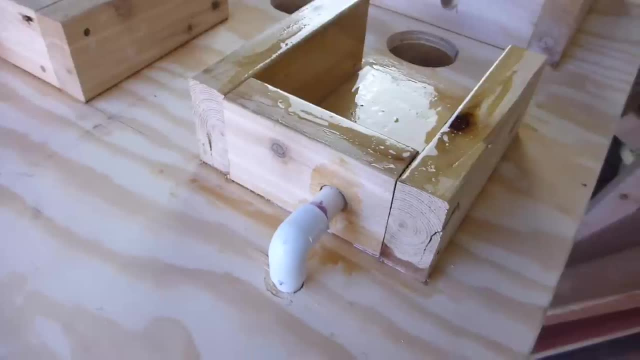 I've never built a wooden boat before, but I think this is how they do it. I've never built a wooden boat before, but I think this is how they do it. The epoxy built up nice thick film and filled in any cracks and holes, so I'm feeling confident that this thing will hold water. 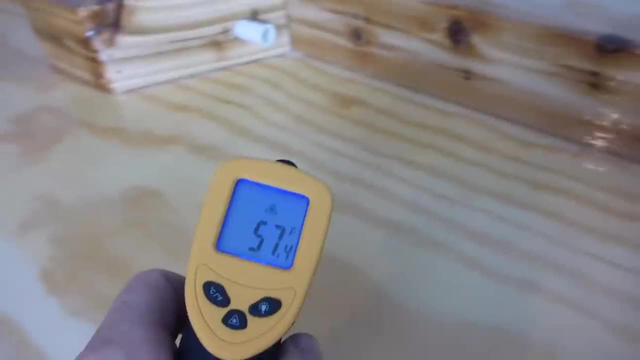 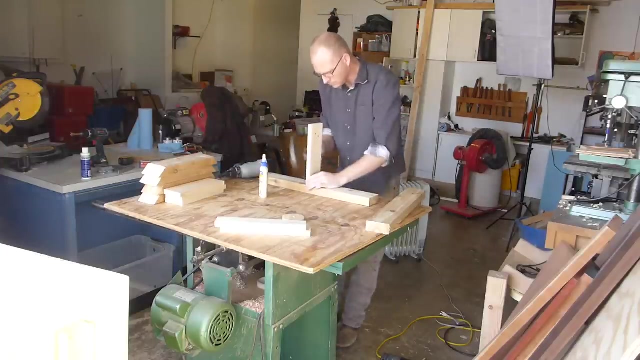 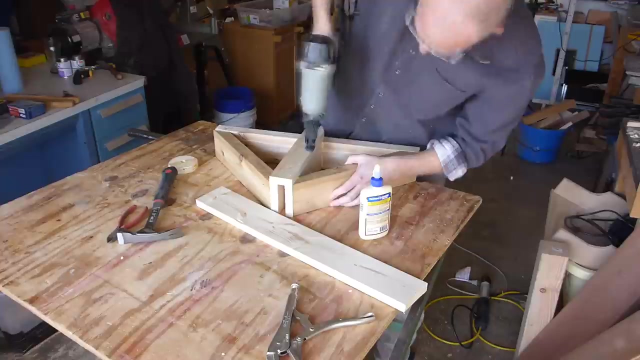 I'm checking the temperature on the epoxy too, just to make sure we are within the recommended range, since it's still a bit chilly outside. While the epoxy was drying, I built the legs which will hold up the display. These are removable so that the display will still fit in my car. 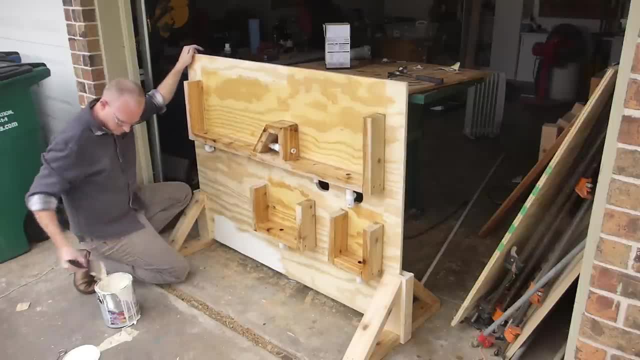 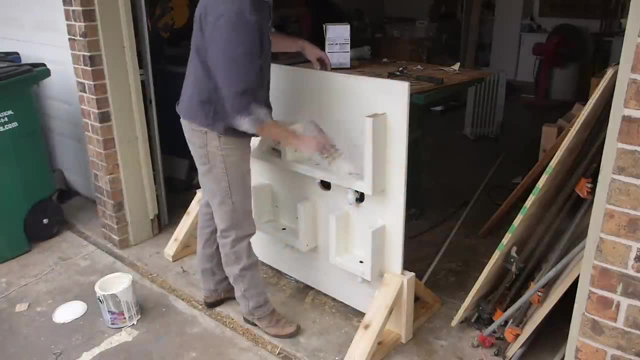 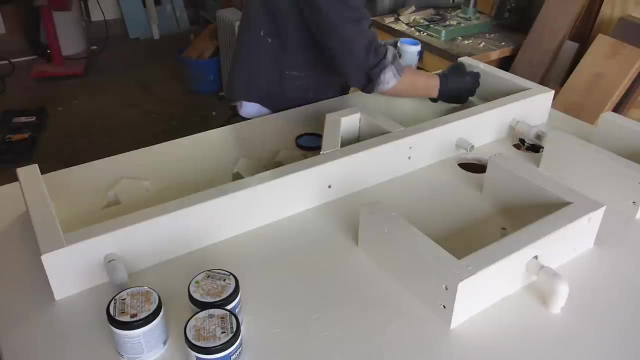 after the epoxy was cured, everything got a coat of exterior latex primer. I figure if this paint can stand being in the weather and the Sun for several years, it can probably stand to sit underwater once or twice a year for a few hours. I got these little sample sizes of colored latex. 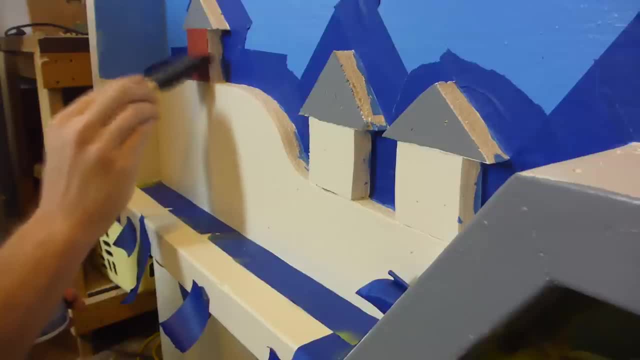 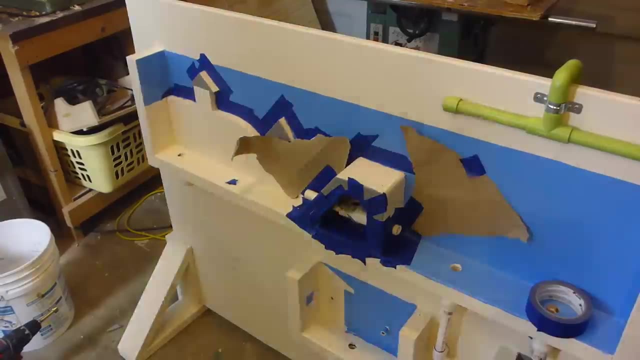 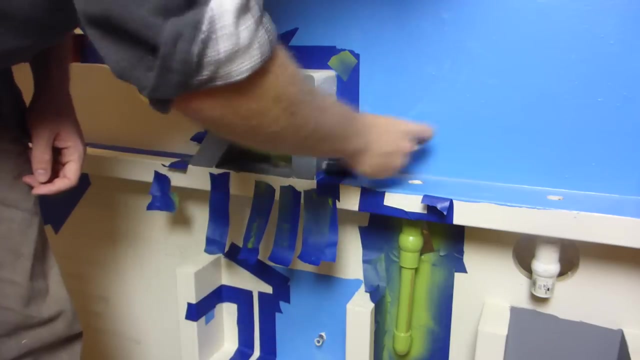 paint. I had no idea you could do this, but these are really cheap, like a few bucks, and the big bucks stores will mix it to whatever color you want and it's really high quality paint. for the PVC pipes, I use spray paint designed for plastic, so I did a lot of masking and a lot 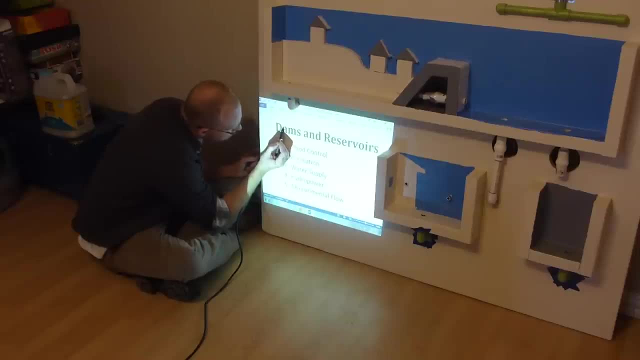 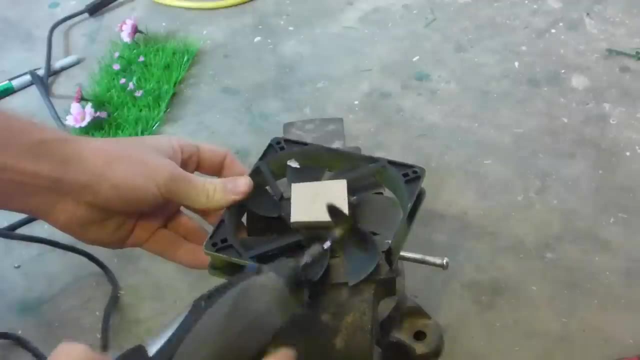 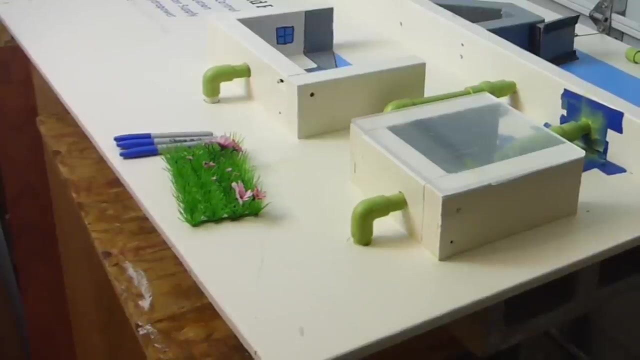 of painting to make it look nice, and then I use a projector to get the lettering on the display and then just sharpies to fill it in. for a few finishing touches, I painted this computer fan green to use as a a hydropower turbine, and I put this fake grass to use as a lawn. 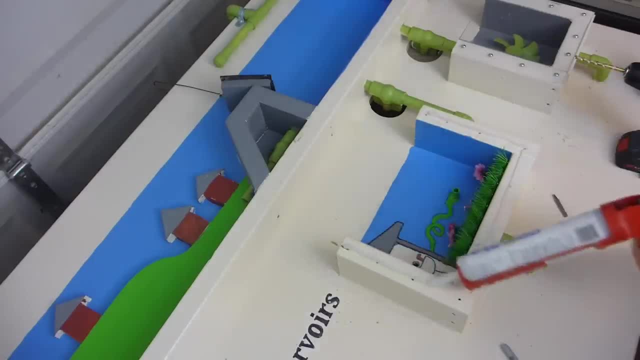 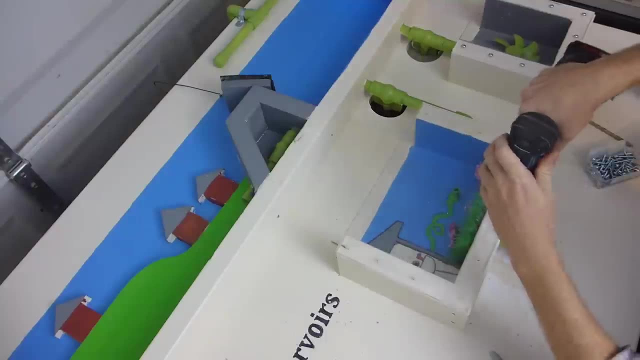 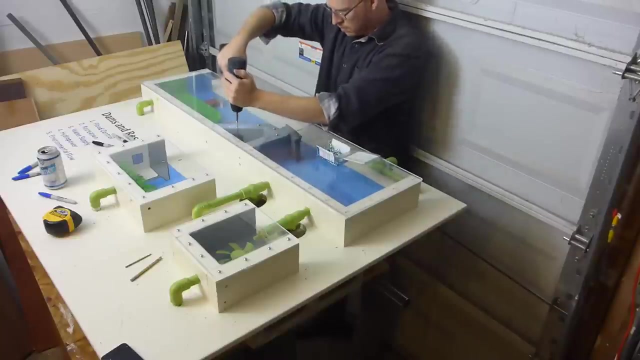 The last step was just to add a nice bead of silicon caulk all the way around the edges and install the acrylic sheets. I pre-drilled all the holes and I used Kreg pocket screws to hold the acrylic down, because they have a nice flat washer head that distributes pressure evenly and will hopefully keep from. 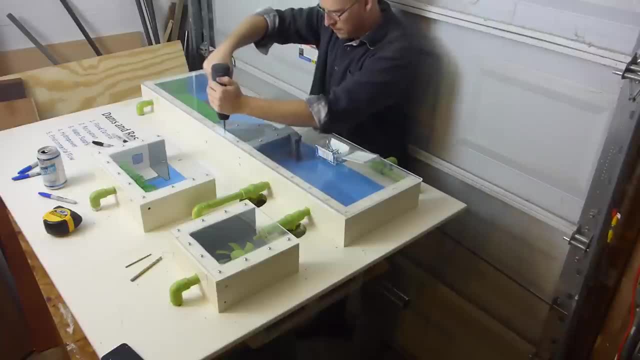 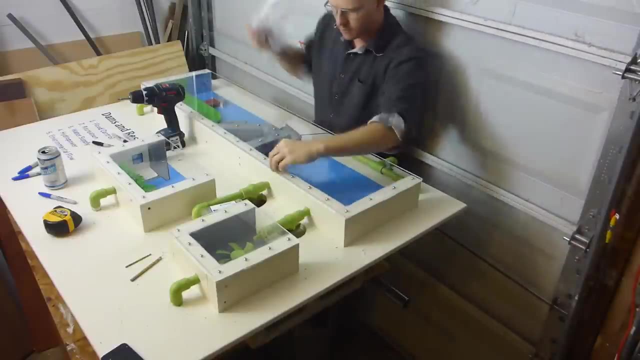 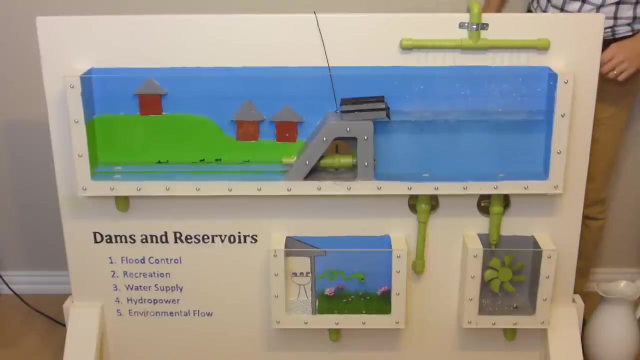 cracking the acrylic, And I set my drill clutch to the lowest setting to make sure I didn't over-tighten anything. This is my favorite part. So here's how the display works. Water is pumped from a tray behind the display to above the lake to simulate rain filling. 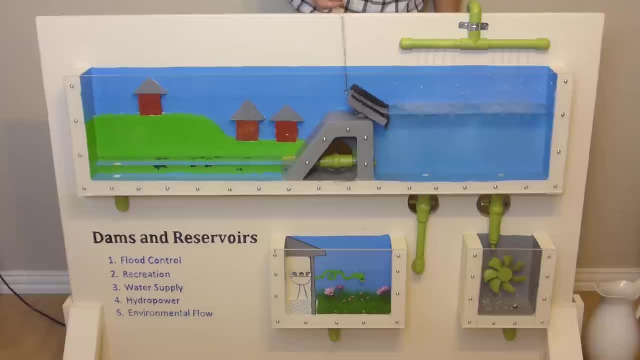 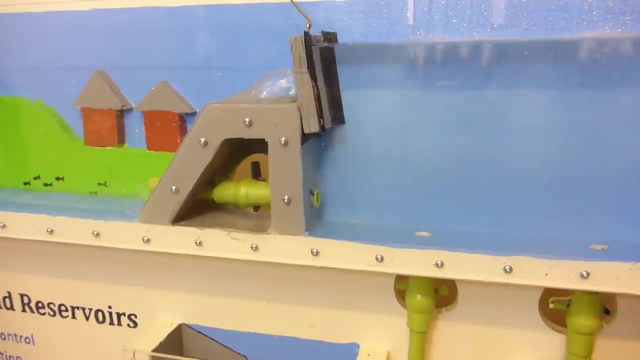 the reservoir. A flood can be simulated by pouring in a pitcher of water. I built a small crest gate. It doesn't seal very well but it gets the point across. There are houses along the bank of the river downstream to show how flooding can affect.